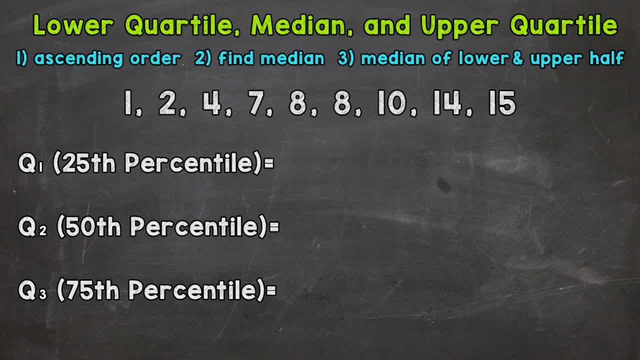 All of this information helps us understand and interpret data. Quartiles are a building block for other topics involving data, so an understanding of this will help you moving forward. We have two examples that we're going to work through. One example will have an odd number of numbers in the data set and the other will have an even number of numbers in the data set. 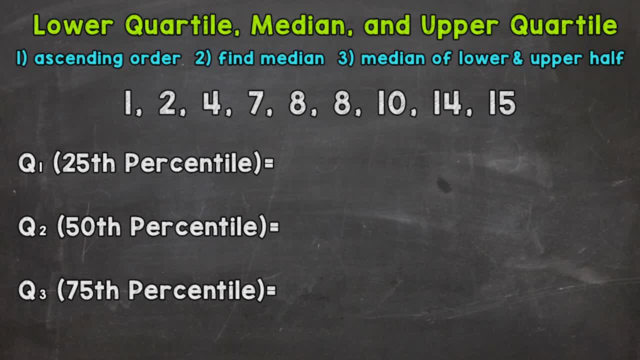 Let's jump into our first example, and in this example we're going to work with a data set with an odd number of numbers. So let's jump into it, and we need to start by ordering our data from least to greatest, so ascending order. 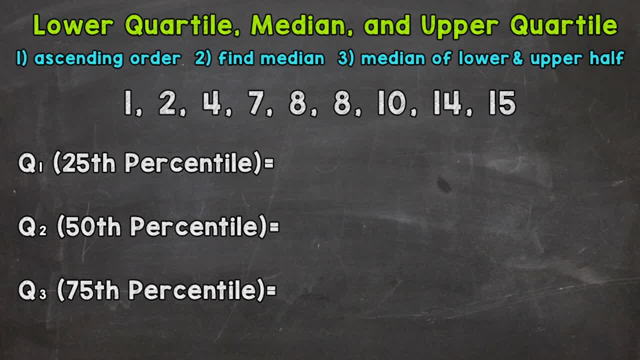 Now, in this example, the data is already in order, but if you're working with a data set that that's not in order, make sure least to greatest or ascending order is the first thing you do. The next step: we need to find the median, also referred to as Q2, which means quartile 2, or the 50th percentile. 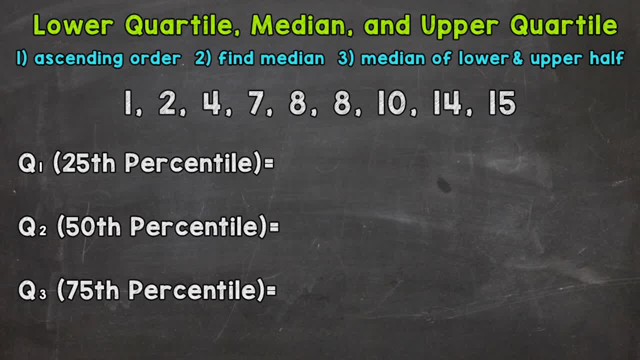 So this is going to be the middle of our data. Now, for this example, we have nine numbers in our data set, So the middle is going to be the fifth percentile. So the middle is going to be the fifth number. That's going to give us four numbers on the left and four numbers on the right. 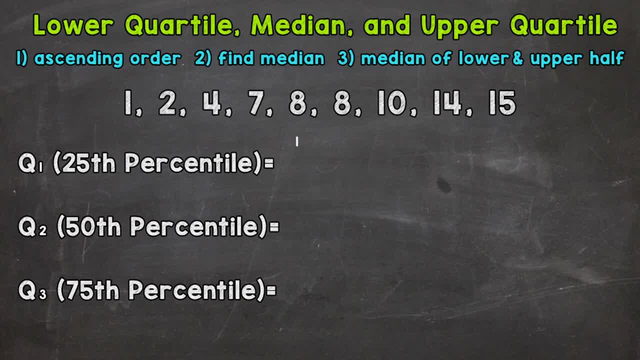 So the fifth number is this: eight. right here That's going to be our median. So let's put eight for quartile 2, or the 50th percentile, or the median. Now that's the middle point. So what we need to do now we need to find the median of the lower half. 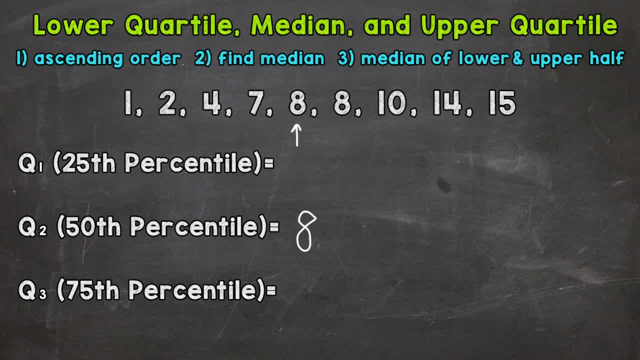 and the median of the eighth And the median of the upper half. The median or middle of the lower half is going to give us the lower quartile And the median of the upper half or middle of the upper half is going to be the upper quartile. 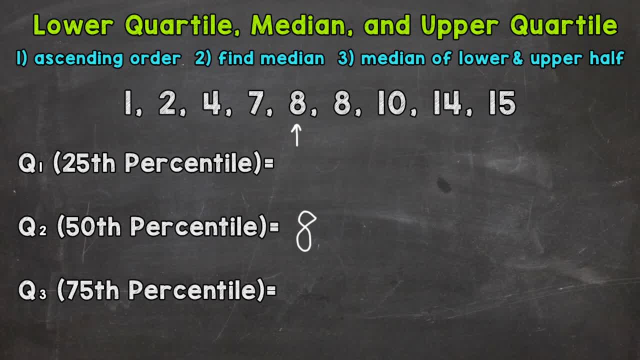 So let's take a look at the lower half first, And we have four numbers here, So we need to find the middle. So we have an even number of numbers within that lower half. We have four numbers, So we don't have a specific number sitting directly in the middle. 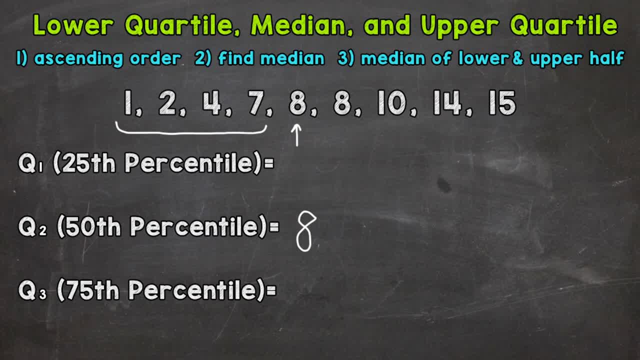 So we're going to have to take a look at the middle two numbers, The two and the four, right here. Now we need to find what's directly in between that two and four. Now we can think this through and we know three is in between two and four. 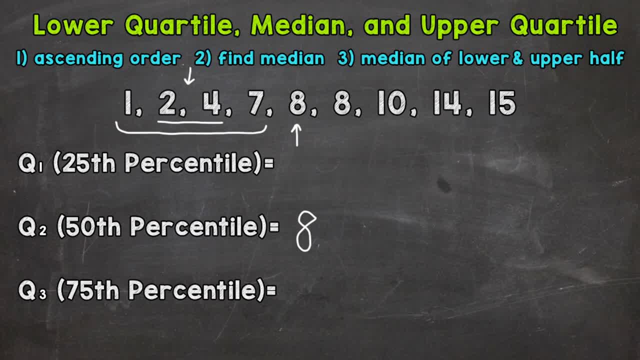 But sometimes it's not going to be that easy to figure out, So we need to do it mathematically. I'll show you how to do that as well, and we'll see if we still get three. So what we need to do if we need the median in between two numbers. 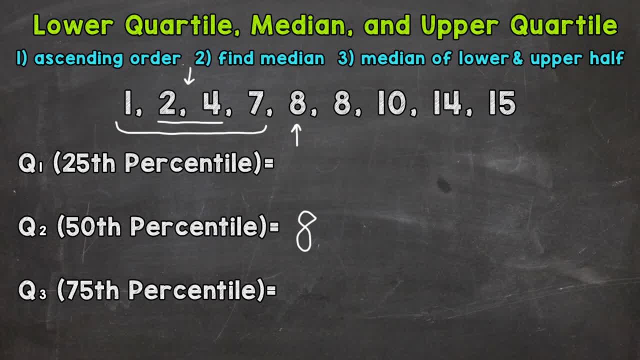 we find the average. So we need to add, then divide by two, So we have two plus four, and then divide by two. That's going to give us our average. So two plus four is six, And six divided by two gives us three. 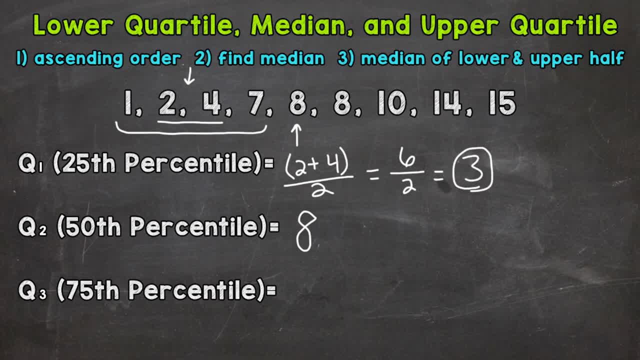 So we still got three. So three is our quartile, one Or lower quartile. Eight is our Q2, to recap, So our median, And now we need to end with finding our upper quartile. So we'll take a look at the upper half. 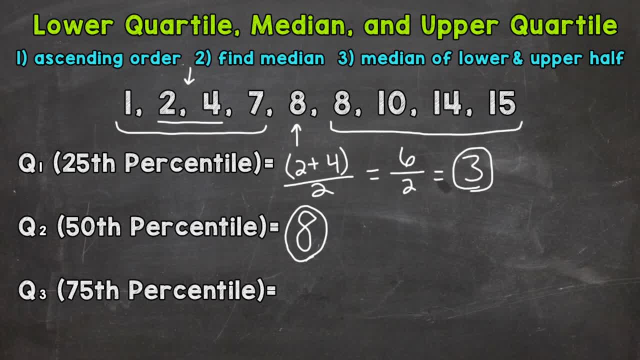 And we have four numbers here, So an even number of numbers. So we need to take a look at the midpoint or middle of our two middle numbers here, So what's going to be in between ten and fourteen? So let's find the average between those two numbers. 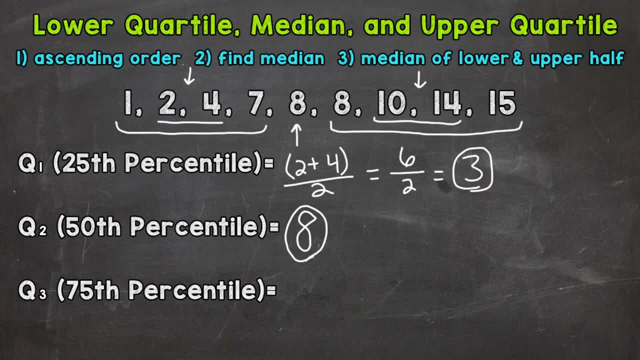 And that's going to give us the median of that upper half. So we do ten plus fourteen And we divide by two to find the average. So ten plus fourteen is twenty-four, And twenty-four divided by two is going to give us twelve. 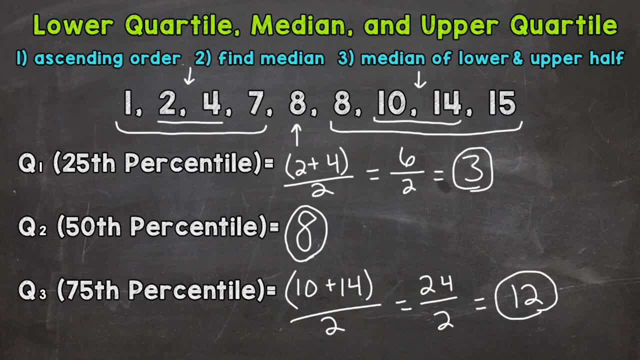 So twelve is going to be our upper quartile. So let's see, Let's split this data set into quarters or four equal pieces to give you a visual of splitting this up. So we know, our twenty-fifth percentile, or lower quartile, is at three. 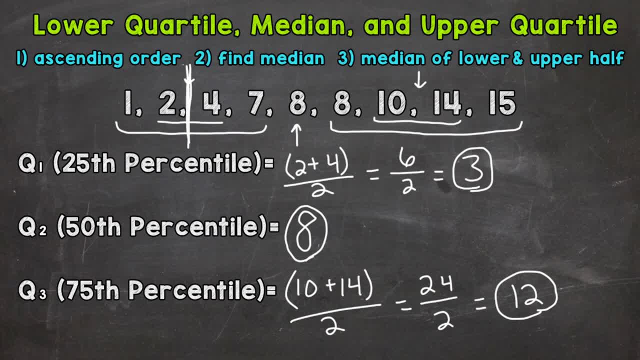 Which is right in between two and four. So I'm going to draw a line. Our median or fiftieth percentile is this: eight, right here. So let's draw a line. And then our upper quartile, or seventy-fifth, Our fifth percentile, is in between the ten and fourteen at twelve. 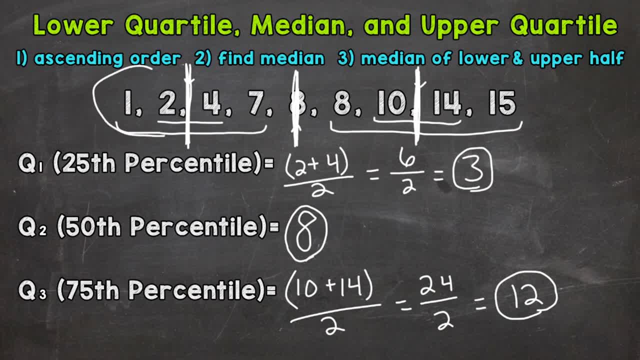 So you can see that we have one, two, three and four equal pieces. That's what quartiles are. We split our data set into four equal pieces Now that we know how to find the lower quartile, median and upper quartile of a data set. 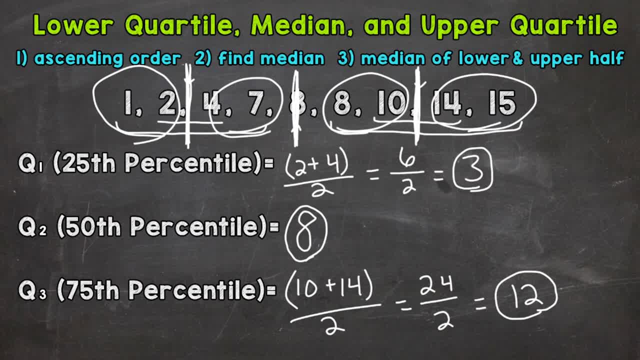 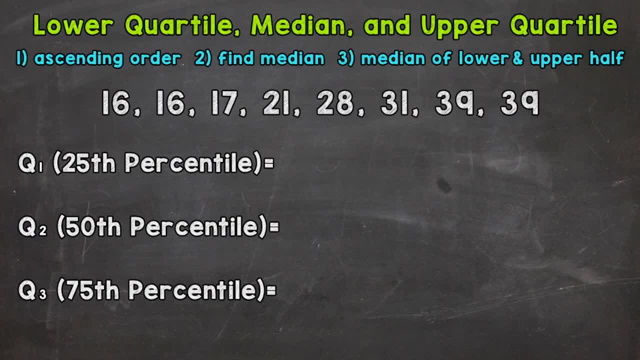 with an odd number of numbers. we're going to take a look at a data set with an even number of numbers, So let's jump into it. In this example, we're going to work with a data set with an even number of numbers. 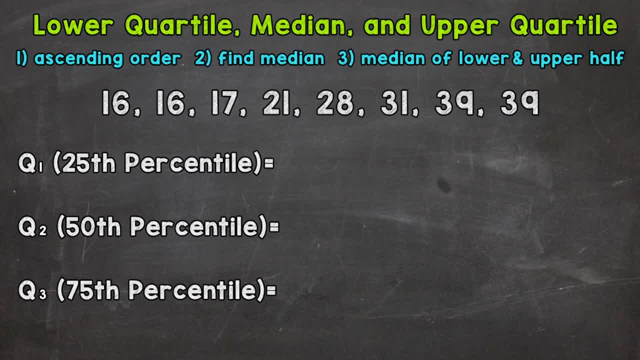 And we need to start by ordering our data from least to greatest, So ascending order. In this example, we are already in order, But if you're working with some numbers that are out of order, you can start with ordering those numbers from least to greatest. 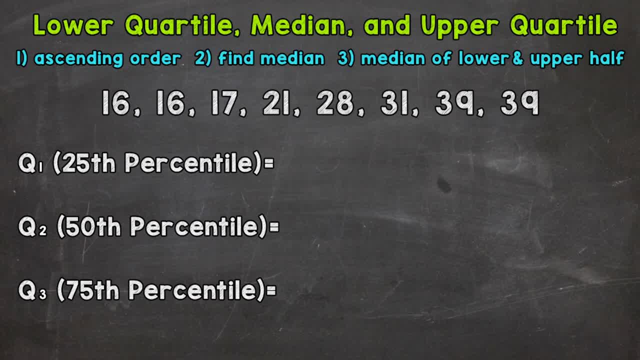 So let's move on to step two, which is find the median. Now we have eight numbers within this data set, So we're going to have four on the left and four on the right. That's going to give us our middle. It's going to be in between the twenty-one and the twenty-eight. 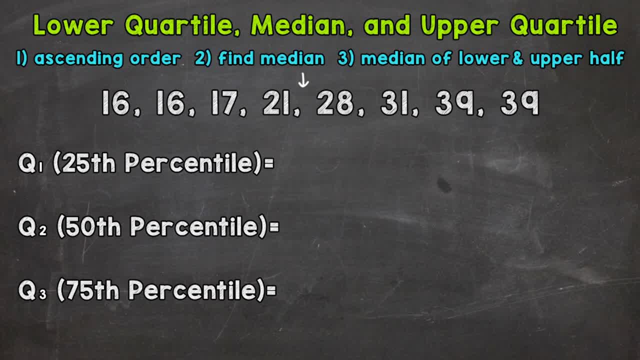 So we need to find the middle between those two numbers, And we can do that by finding the average. So let's come down to where it says Q2, which stands for quartile two, which is the same thing as the median. It's the fiftieth percentile. 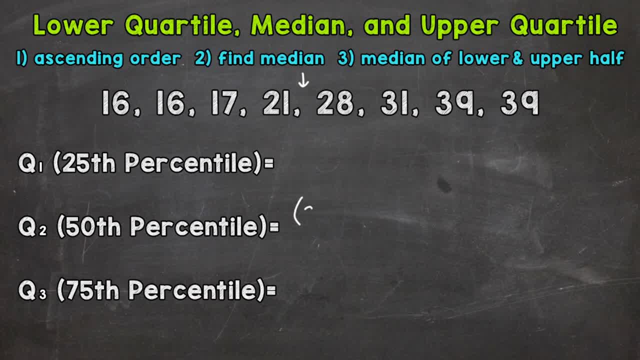 So to find the average we need to add those numbers, Twenty-one plus twenty-eight, And then divide by two. So twenty-one plus twenty-eight gives us forty-nine, And forty-nine divided by two is going to give us twenty-four and five-tenths. 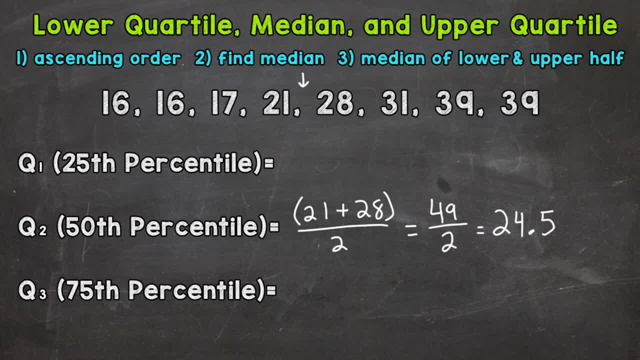 Or twenty-four and a half. That's going to be our median. That's the middle point of our data set there. So once we have our median, we need to find the median of the lower half and median of the upper half. The median or middle of the lower half is going to be the lower quartile. 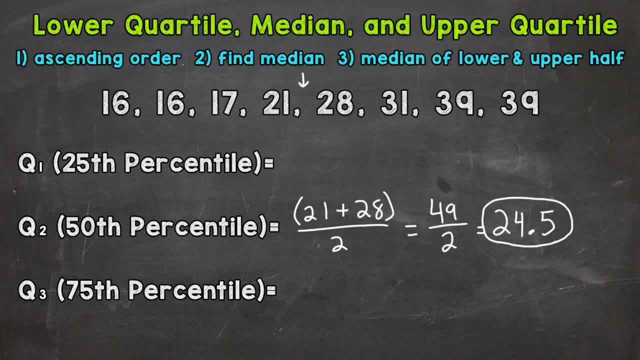 And then the median or middle of the upper half is going to be the upper quartile. So let's do the lower half first, So the lower four numbers. We need to find the middle of those lower four numbers And since we have an even number of numbers there, 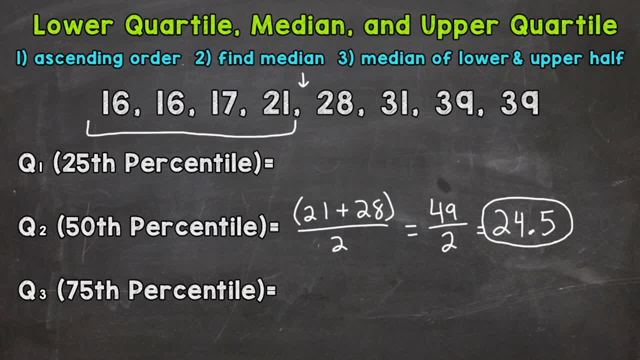 we don't have a number sitting directly in the middle, So we're going to need to take a look at the two numbers in the middle and find what's in between. That's going to give us our median Again, because we don't have one specific number sitting in the middle there. 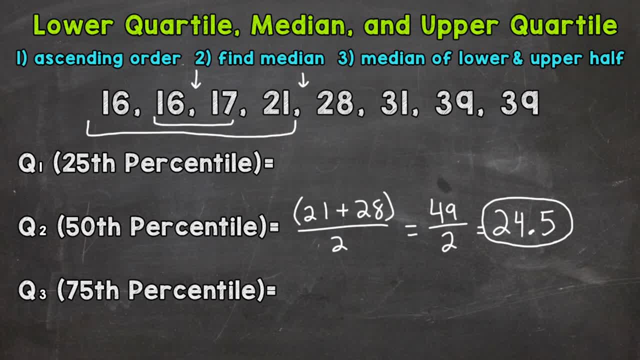 so we need to take a look at the two in the middle and find what's in between And, just like the median, we can do that by finding the average. Or, in the case of this one, we can probably think it through and we know that sixteen and a half is in between sixteen and seventeen. 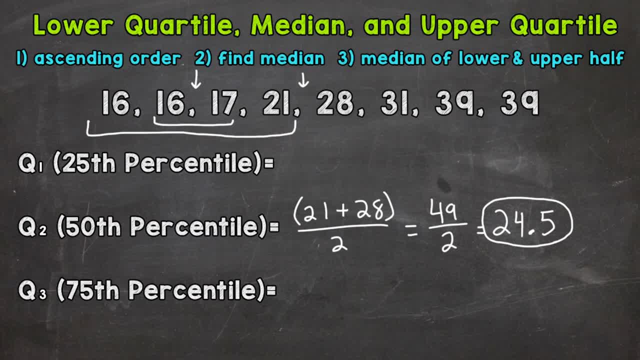 But let's solve it mathematically as well. So again: average, add sixteen plus seventeen and then divide by two. So sixteen plus seventeen is going to give us thirty-three. Divide it by two and we get sixteen and five-tenths. 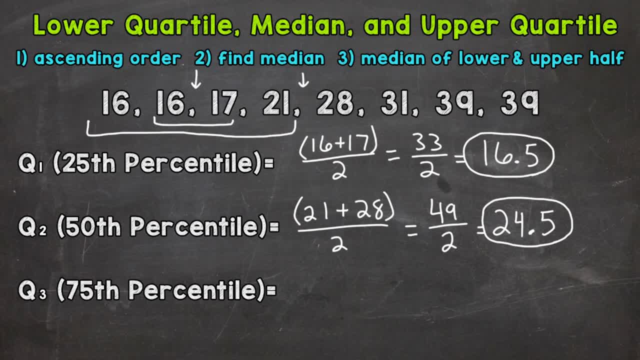 or sixteen and a half. That's going to give us our lower quartile. So that's the twenty-five percent mark within our data set there, the twenty-fifth percentile. So once we have that we can do the upper quartile. 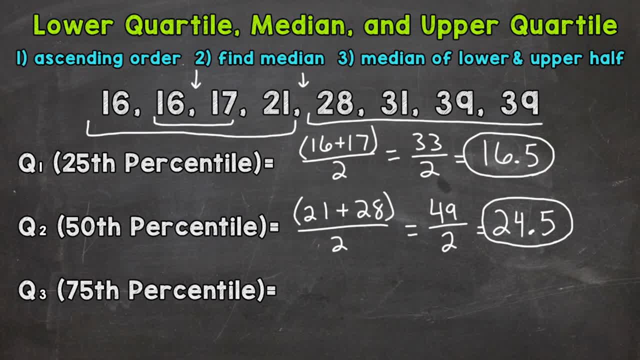 So let's take a look at the upper half and find the middle or median of that upper half. Now we have four numbers, again an even number of numbers, so we're not going to have one specific number sitting in the middle. 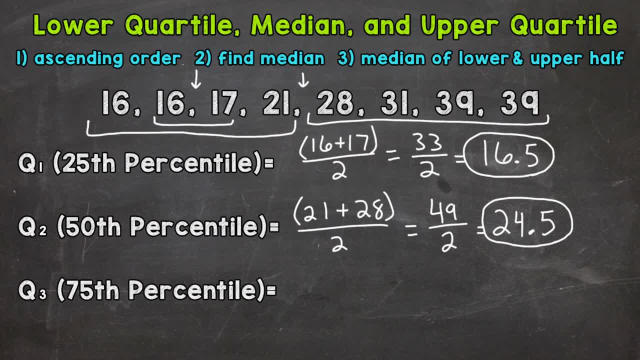 We're going to take a look at the two middle numbers, which thirty-one and thirty-nine, and find the midpoint between those two. That's going to give us our median of that upper half. And we can do that by finding the average. 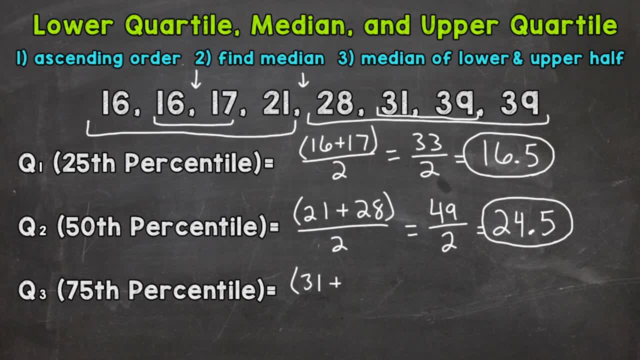 So add thirty-one plus thirty-nine divided by two, Thirty-one plus thirty-nine is going to give us seventy. Seventy divided by two gives us thirty-five, So thirty-five is going to be the upper quartile. It's the seventy-five percent mark within our data. 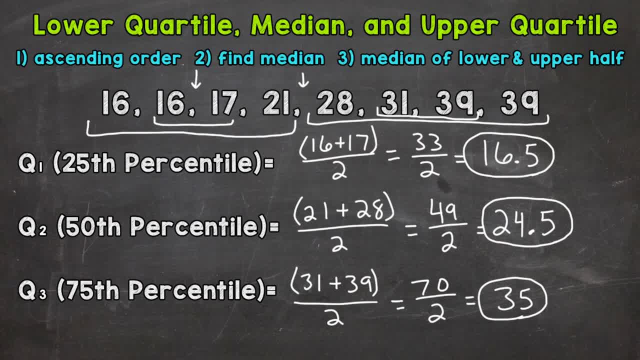 the seventy-fifth percentile. So those are our quartiles. The lower quartile is sixteen and a half, that's the twenty-fifth percentile. Then we have the median, which is twenty-four and a half, that's the fiftieth percentile. 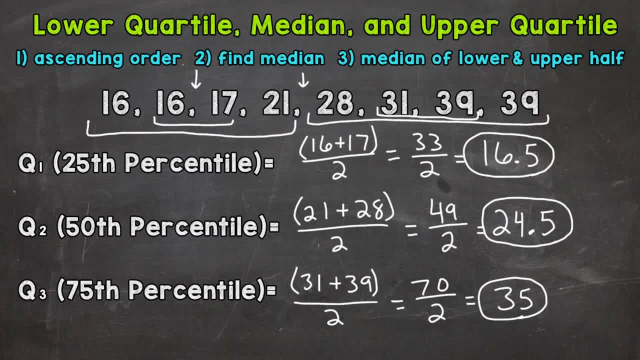 the middle of our data set And then for our upper quartile we have thirty-five, so that's the seventy-fifth percentile. I'm going to draw some lines within our data set there so we can visualize where these quartiles are. 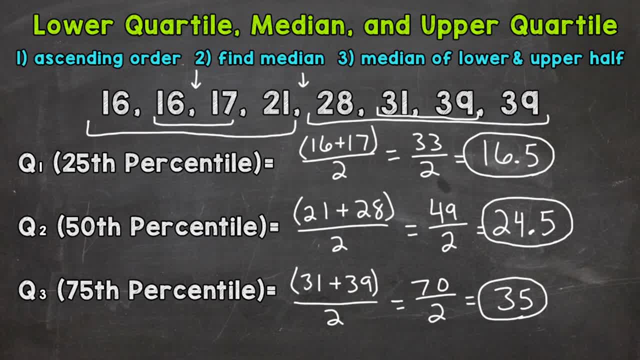 and how it breaks our data into four equal parts. So sixteen and a half is going to be right here, Right in between that sixteen and seventeen that we talked about earlier. The median, which is the middle point, is right here, in between the twenty-one and twenty-eight. 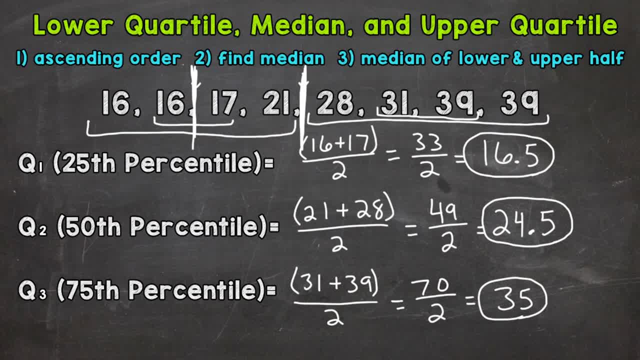 like we talked about earlier. And then we have our upper quartile in between the thirty-one and the thirty-nine. So you can see that we have one, two, three and four equal pieces. This line right here represents the twenty-fifth percentile. 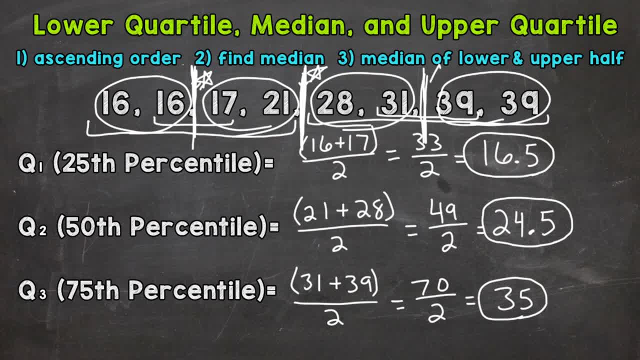 This line is the fiftieth and then this is the seventy-fifth. So there you have it. There's how you find the lower quartile, the median and the upper quartile. I hope that helped. Thanks so much for watching.